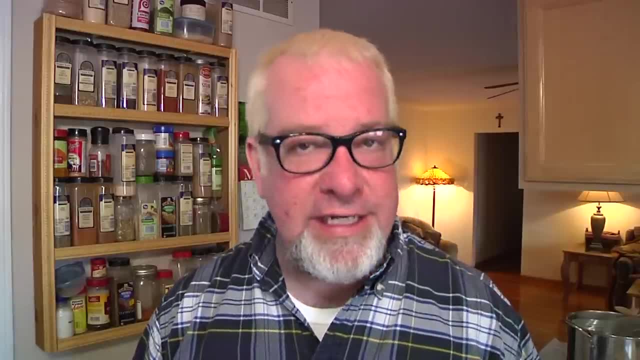 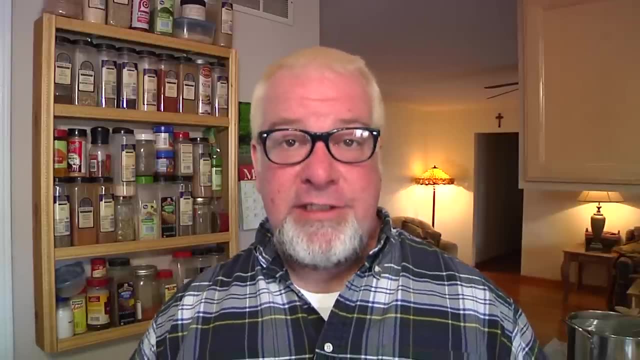 this. This is super, super basic, easy soap. You only need really three things: water, lye and a fat, And that's it. It's just getting your stuff right And we're going to show you how to do. 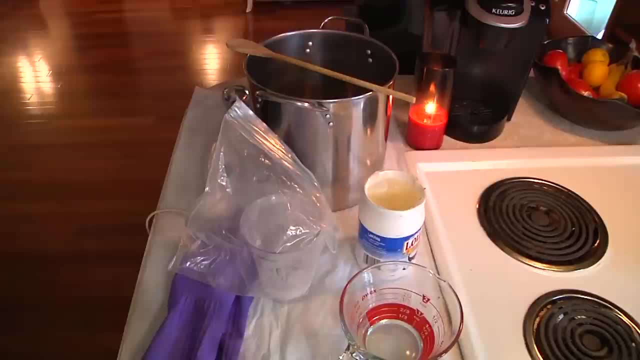 that right now. So here we go. All right, So stuff we're going to need to make this very, very basic soap. The ingredients are super simple. There's three ingredients. You're going to need eight ounces of filtered water And for our fat, we're actually going to. 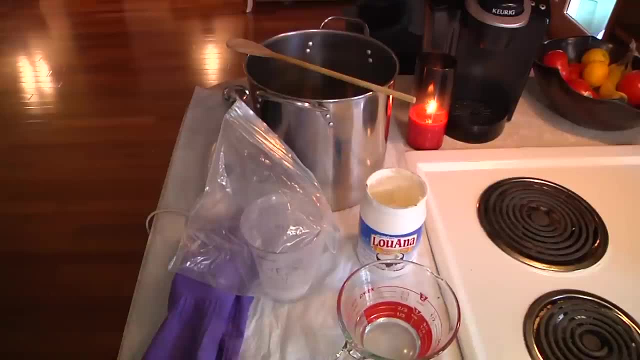 use 22 ounces of coconut oil. We like the coconut oil for a lot of different reasons. One is it's very good for your skin and it has a very low melting point, So it's easy to use. And for the lye, which is also called sodium hydroxide- for those techno people out there, it is. 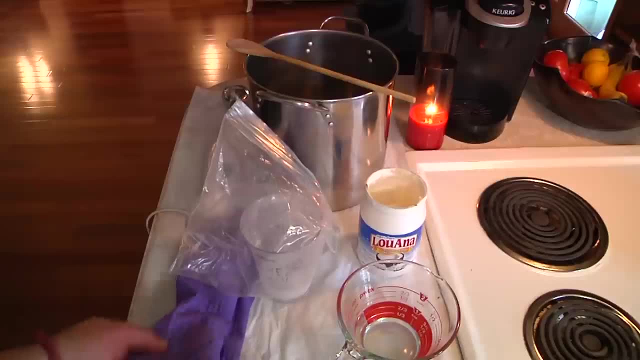 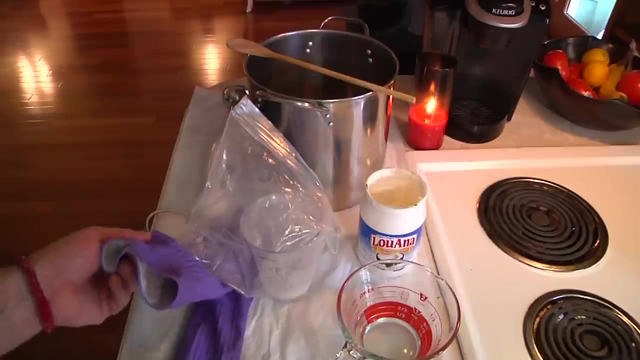 2.8 ounces. You need some gloves Lye when the chemical reaction is going to happen. it's going to get very hot and it can burn you, So you've got to be careful. So we use the rubber gloves. 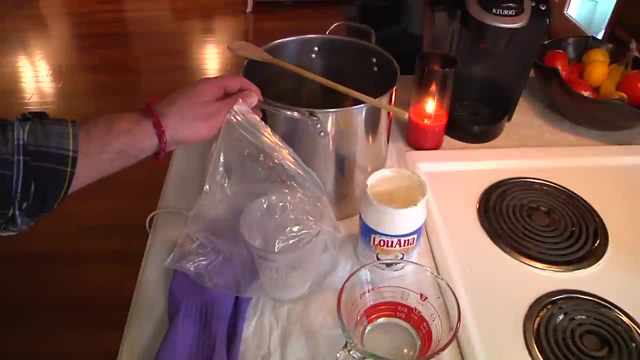 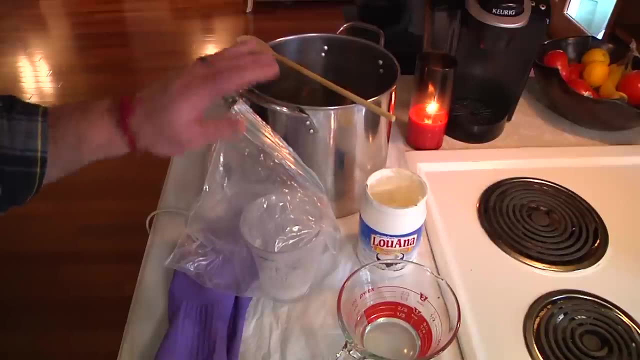 Okay, Now one other thing that's very important: the pot that you're going to make it in, you need to make it stainless steel And you can use other materials, but I do not recommend it. No, no, no, no. Glass can actually the heat difference when the chemical reaction is. 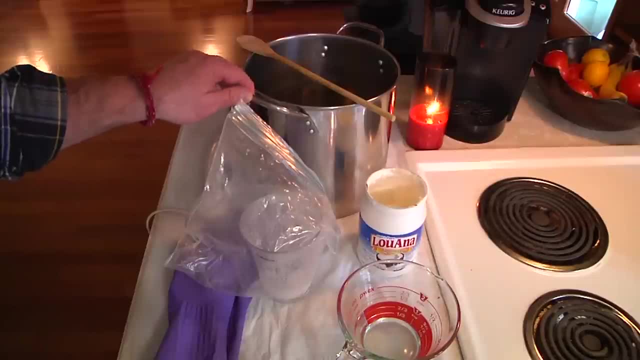 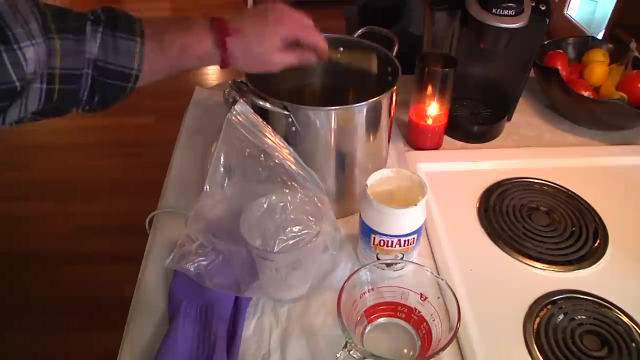 happening can cause your glass To break. Aluminum will actually have a chemical reaction. It starts to melt and degrade and it's it's bad, bad, bad all the way around. So I just recommend that you use stainless steel. Old faithful works every time. One other thing: that we use a basic wooden spoon to stir with. 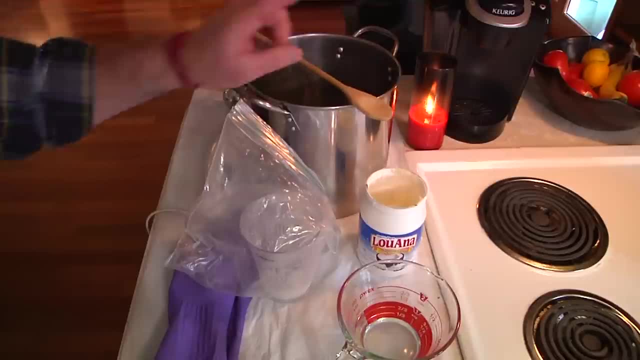 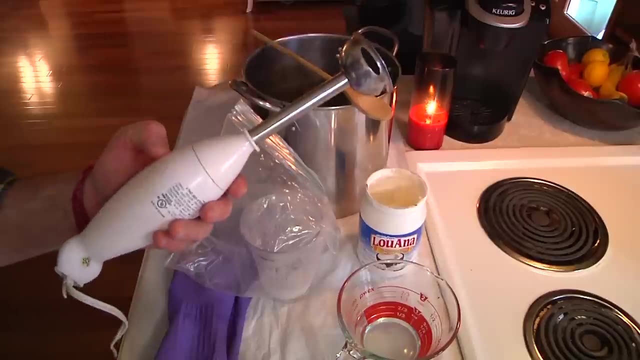 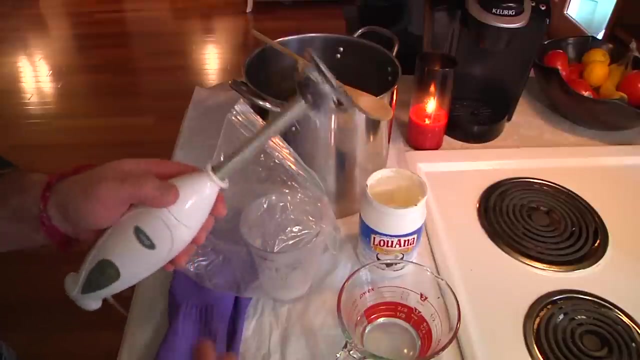 You can make the entire soap recipe with just this, but if you get one of these stick blenders, this is going to help you so, so much When it comes to the process of saponification that I will show you. uh well, my wife and I, once again, 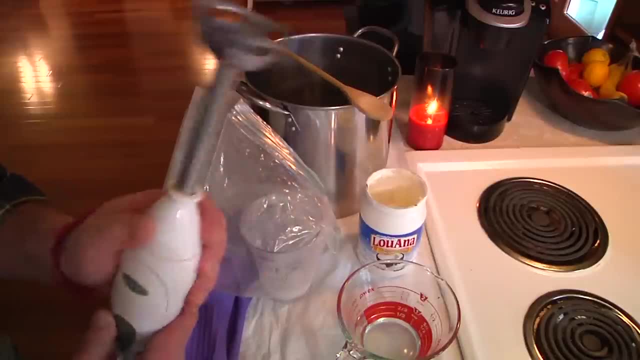 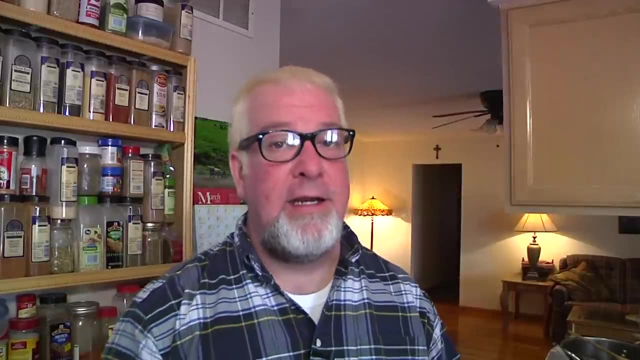 get it right, Brad, that we'll show you later. Um, but this helps saponify and get what's called trace much, much faster. All right, One last thing that I nearly forgot, And it would have been kind of funny, uh. 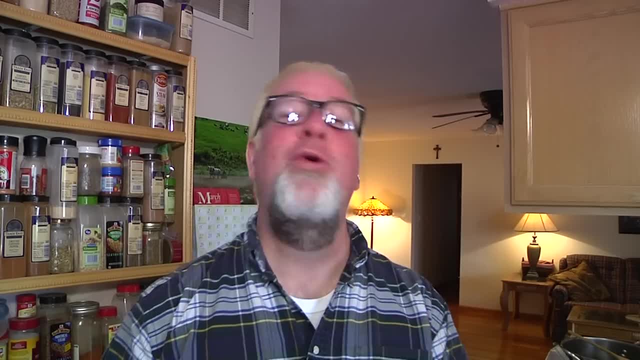 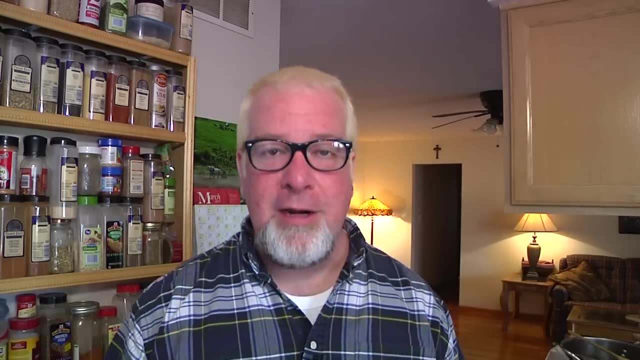 if we were filming, and I'm running around looking for this crucial item, and that's something to put your soap in dummy. So we got these little trays- uh, that that were only a buck. We got them at the dollar store and and it's a mold. 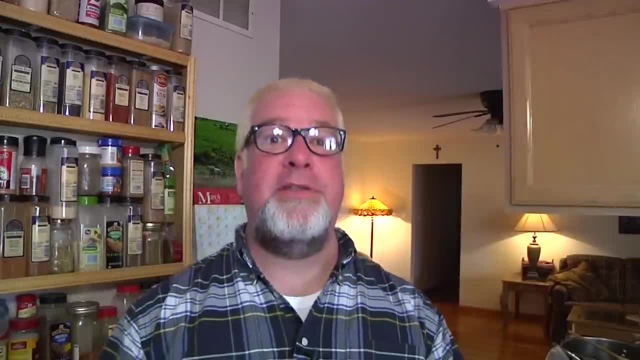 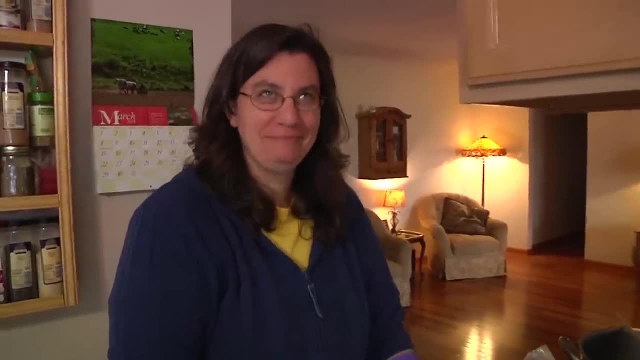 You're going to pour your soap in here. Kind of important to have something to put your soap in Jeez. So here's my lovely waif of a wife. She's so delightful and she's really irritated with me right now. 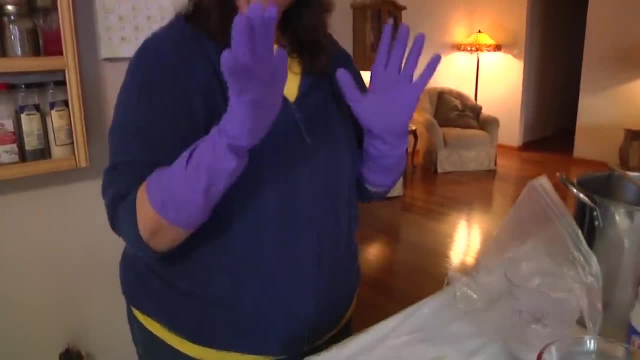 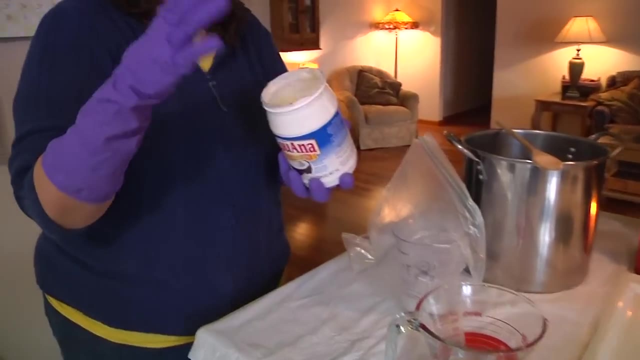 We're going to make soap, aren't we? So she's gloved up, gloved up, ready to rock. Okay, First things first. What are we doing? It's going to melt some oil. melt, the oil has to get to at least a hundred degrees. a hundred degrees. 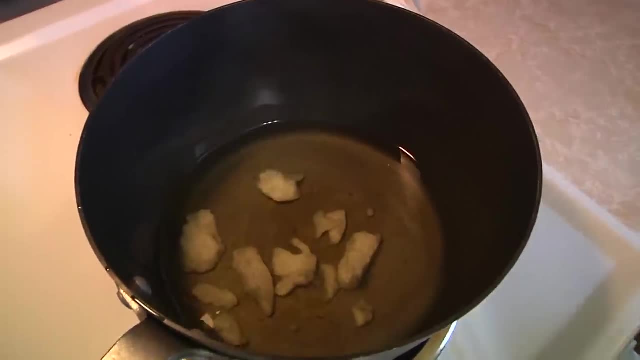 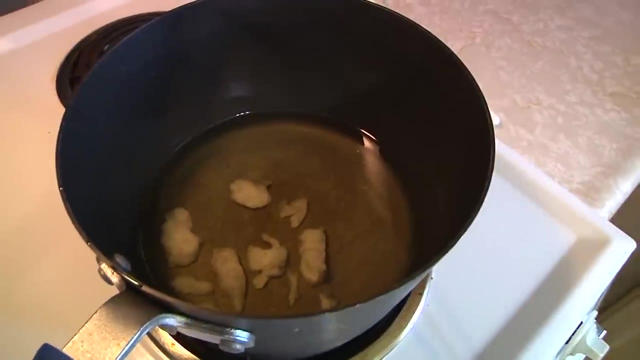 Melting the oil. Aye, aye, sir, Here we go. Okay, Our coconut oil is nearly melted. And one note on the fat. This is our fat in the recipe And basically you can use any old kind of oil you want. You can use vegetable oil. 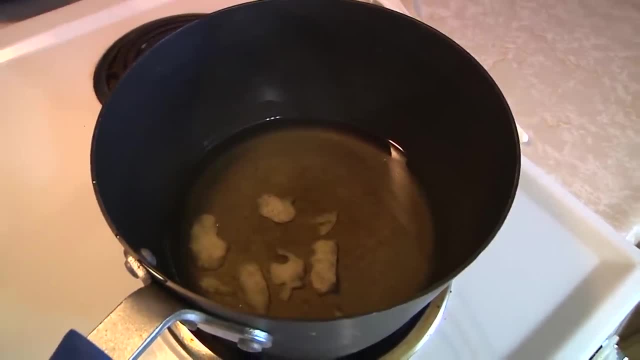 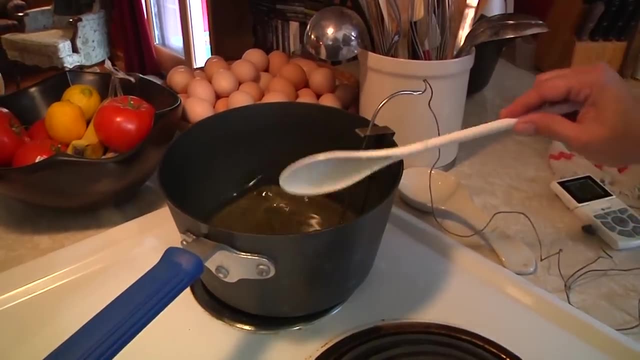 You could use fat for hunters out there who process animals. You can render that fat and make soap with it. It can be anything, Just need the fat, like me All right. Now our, our fat, our coconut oil is completely melted and it's a hundred degrees. 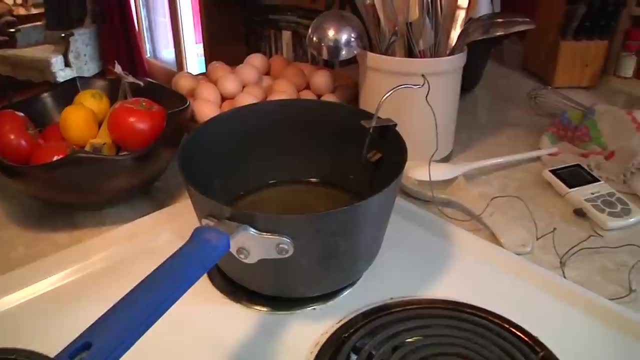 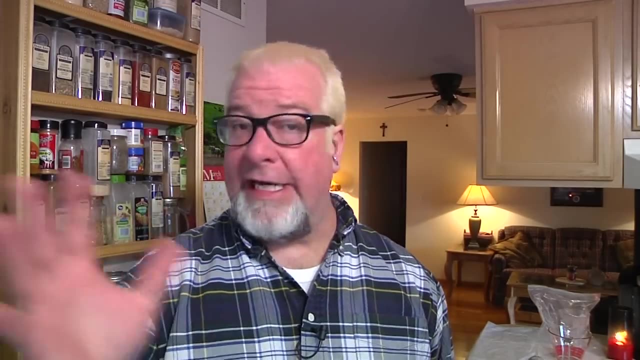 You just don't want it to go over 120 degrees for the next process, where we're going to go ahead and mix it up. All right, One precaution: when you're dealing with lye, it can burn you, right. We all know this. Well, here is the quick way to kill that burn. 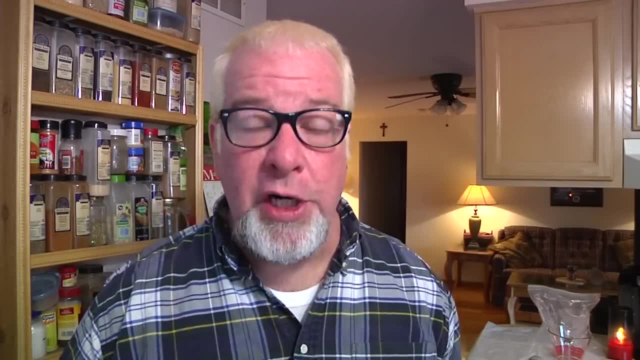 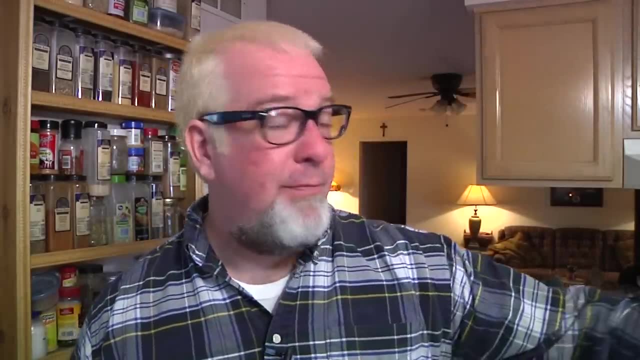 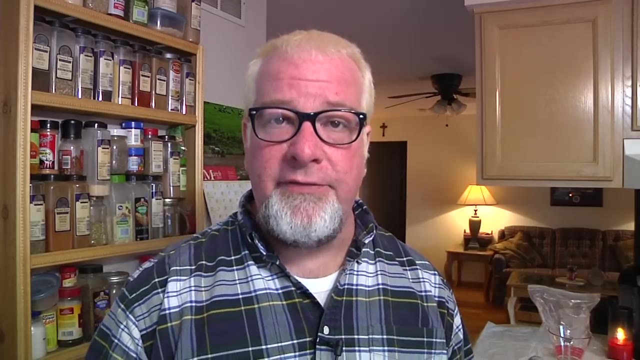 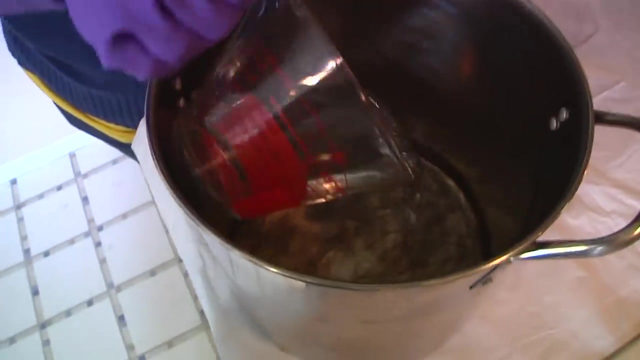 If you get some of it on you and it's, it's burning you. this right here: bang regular old vinegar, pour this onto that, burn onto the lye and it will stop the burn. Uh, it's just helpful to keep it around when you're making this stuff. Uh, good tip, All right, Next up, we're going to go ahead and put our water into our pot and then we are going to add our lye. 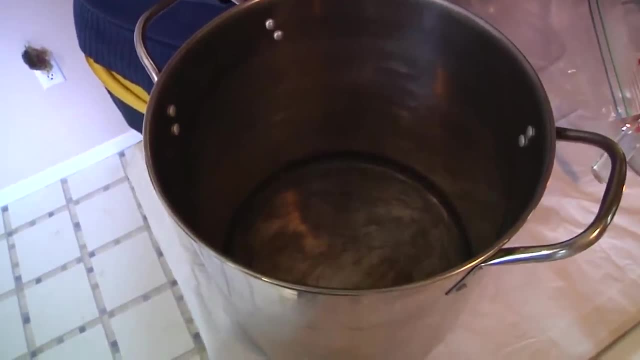 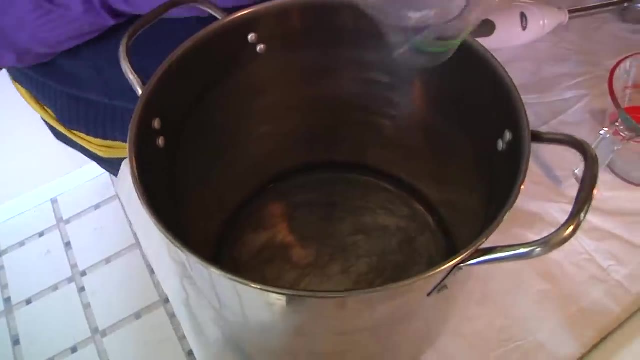 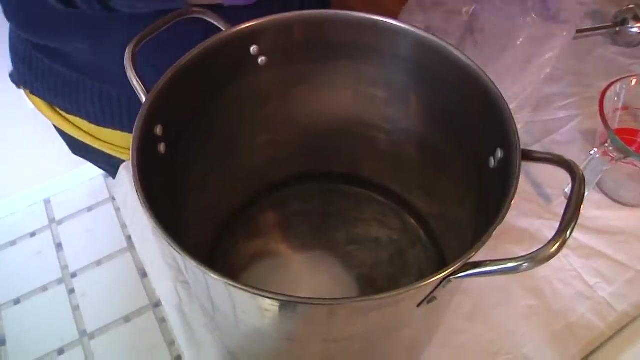 And this is an important- uh well, an important- process is because you don't want the uh lye to just uh have a chemical reaction too quick. You don't want it to splash up on you. So in goes the lye. Notice the gloves. You're very, very careful. Now what's going to happen is this is going to heat up. 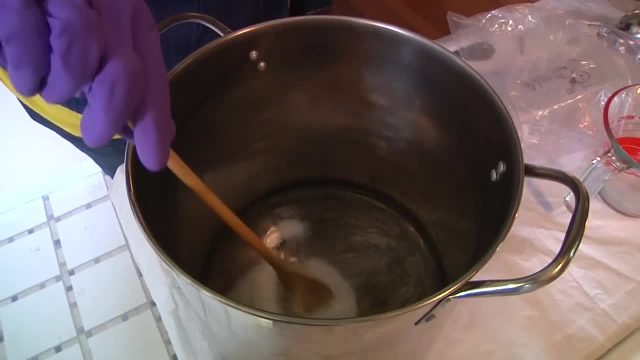 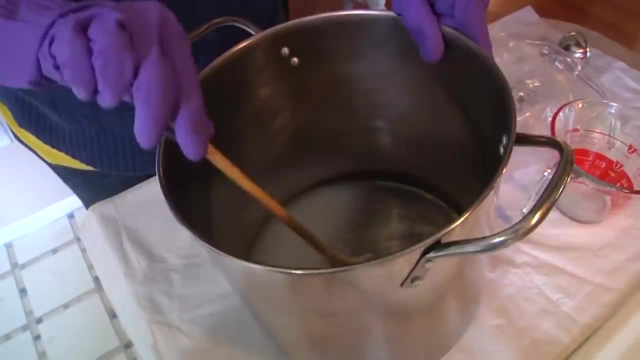 The chemical reaction. when the lye and the water come together, it's going to heat up Now. it's also very, very important that you're doing this in an area that is well ventilated, because it will give off gas that is nasty, nasty, nasty and can hurt your lungs badly. 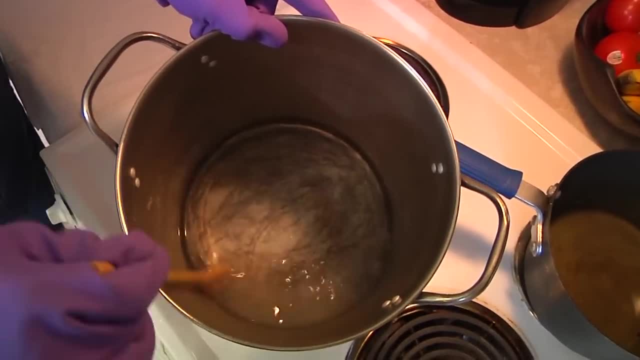 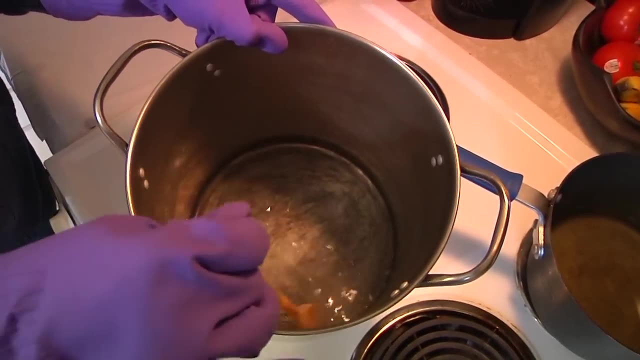 Do not breathe this, Okay, So now what we're doing is we're wanting to make sure that the lye is completely dissolved in the water, and we're going to wait until the fumes- the gas is coming off- are done, And we want this to get. 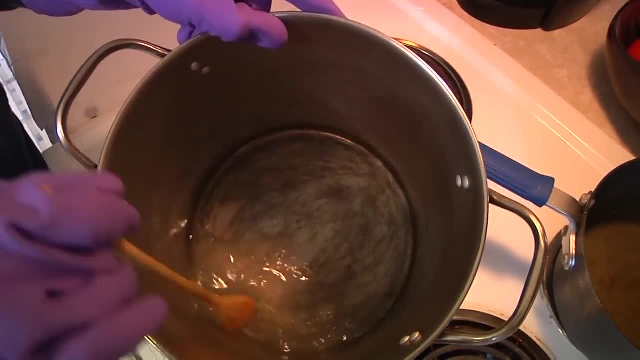 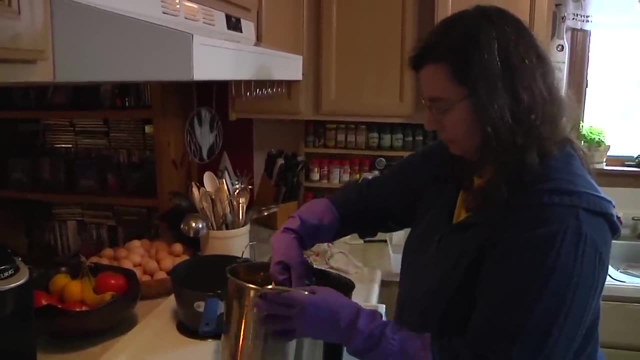 down in temperature to about 120 degrees. Okay, So next up, we, we basically what we're trying to do is get the two, uh, the fat in our lye with the water at around the same temperature, at, you know, a hundred to 120 degrees. 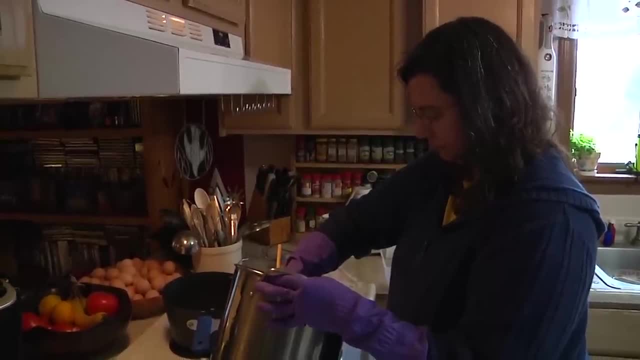 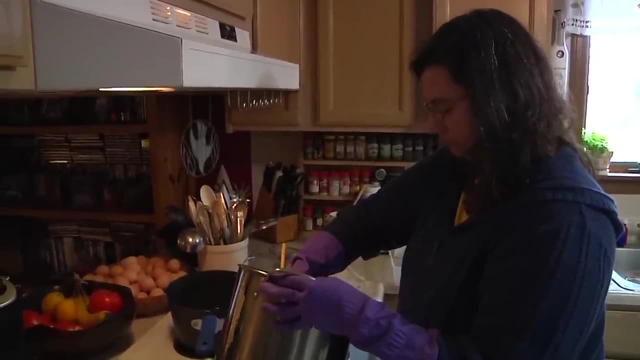 And the closer you get to the same temperature, the easier it will be for, uh, the saponification to happen, the actual making of soap chemically. So we're going to, We're going to go ahead and put these two together. 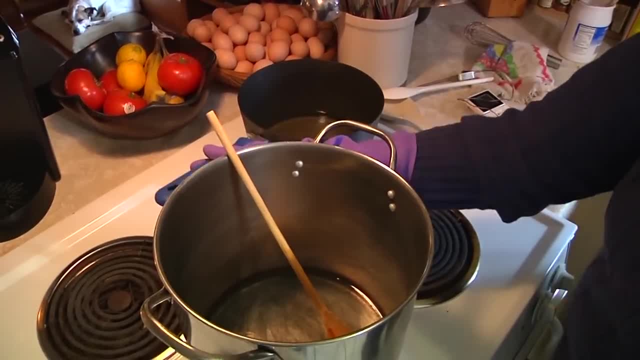 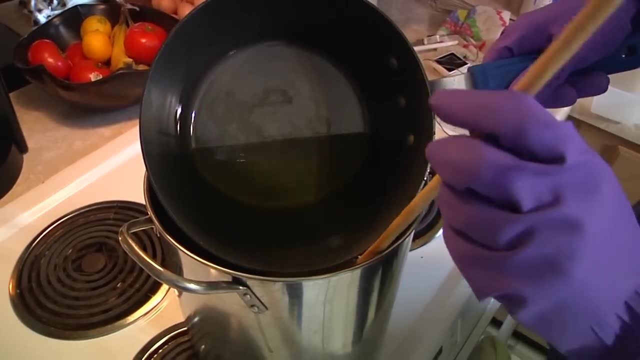 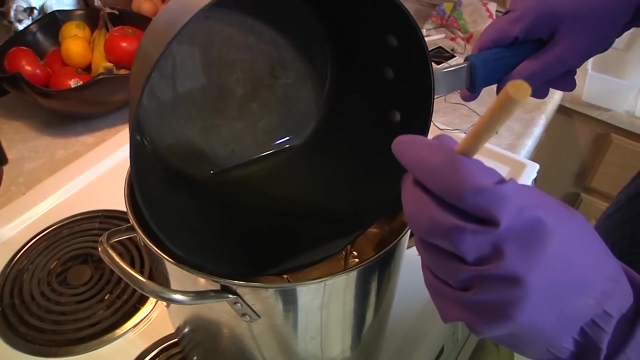 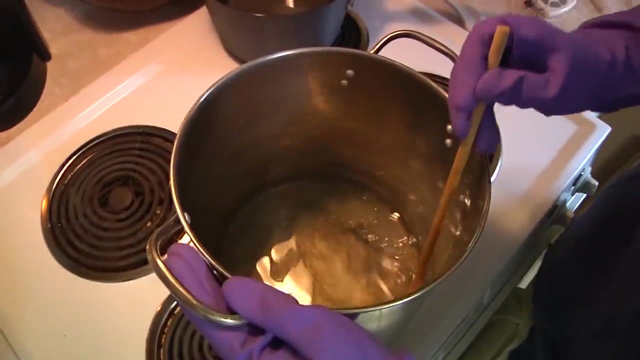 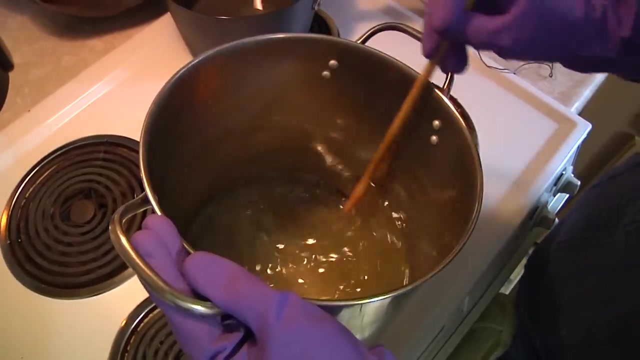 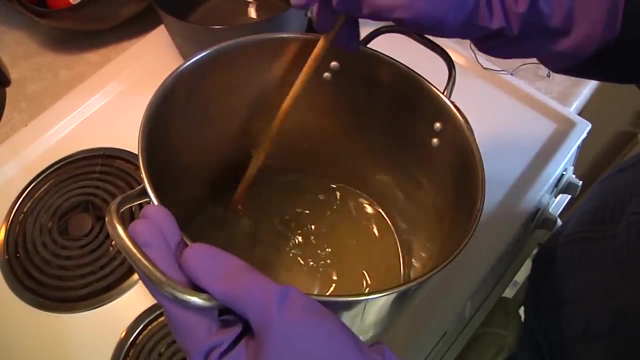 So the fat is going to go into the lye and the water very carefully, extremely carefully. You splash that lie on you and it will burn you. All right, Now we're mixing. what is going to happen Now is, as that is agitated in its- in its, uh, stainless steel pot, of course, because if we used aluminum we'd be cotton headed, ninny muggins, because I already told you can't use aluminum. but it's going to start to saponify. 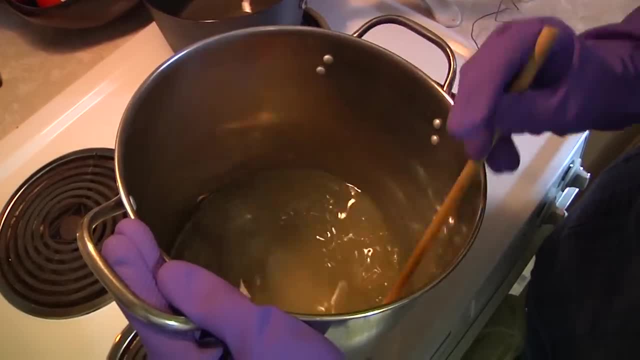 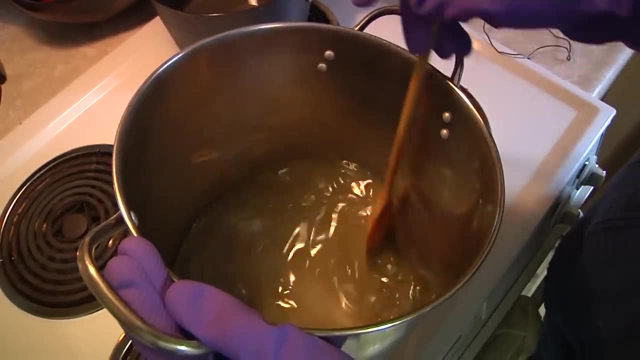 And what that's going to be is there's a chemical reaction that's happening, that all of those things are coming together and it is no longer going to be fat involved and no longer going to be water and no longer going to be lye- all individual things. 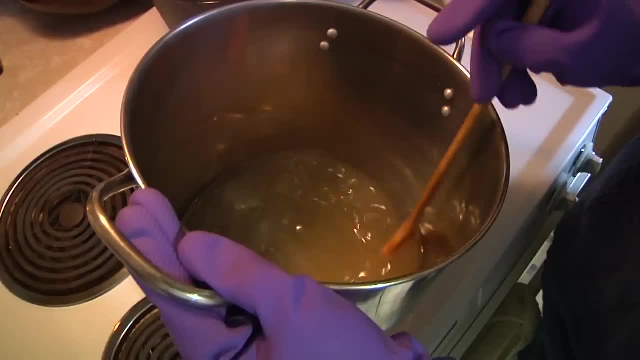 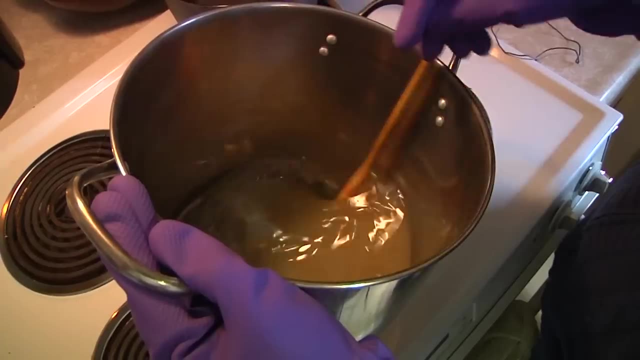 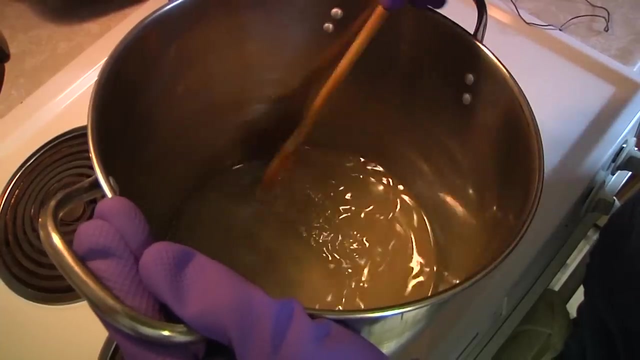 It's going to make one product of soap. Now what what is also going to happen is what we're looking for- is it's going to start to thicken up on us and that's going to cause what's called trace, where the viscosity of this- right now this liquid- is very runny. 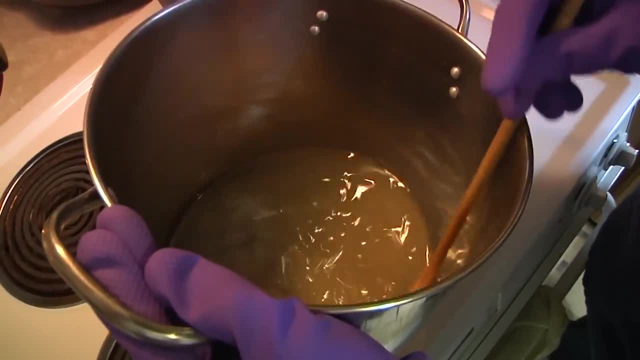 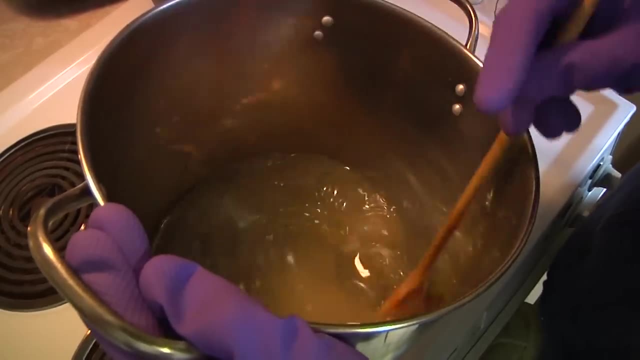 It's very water, like it's going to start to thicken up and it will make what's called trace and that it kind of just will show you what it is. but it makes it a little more gloopy and leaves kind of trails behind. 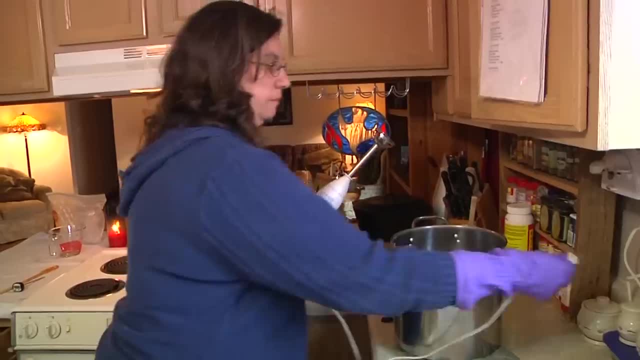 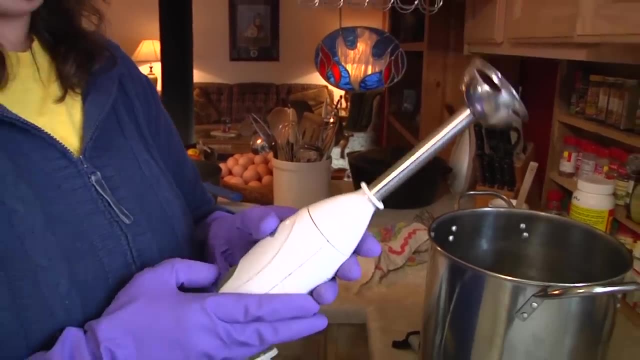 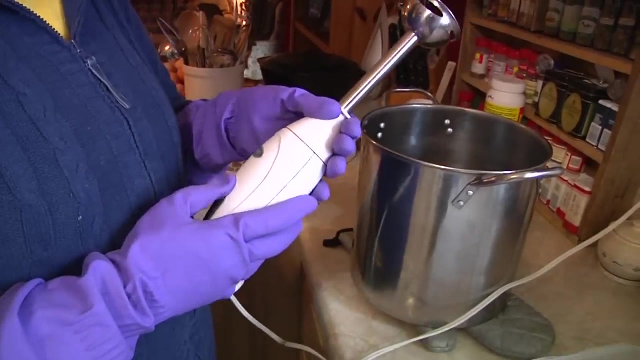 Uh, your spoon when you're mixing it. now, in the interest of saving time- because we do have high tech tools like our blender stick, blender thingamabobber- we're going to go ahead and ditch that wooden spoon. You can make the soap with just the wooden spoon, but this is going to take a lot less time. 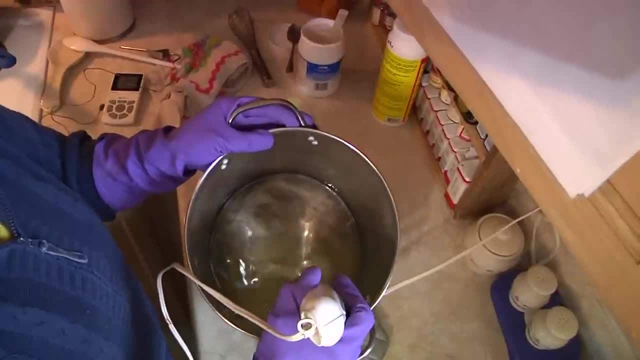 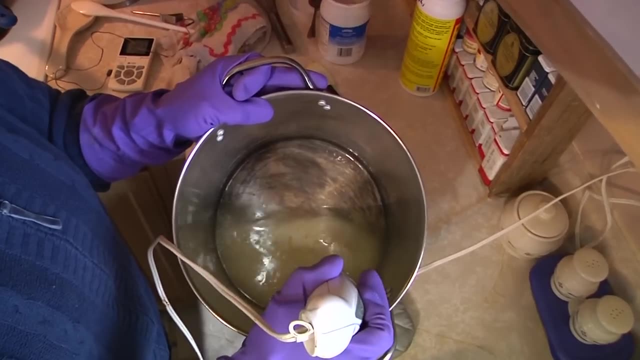 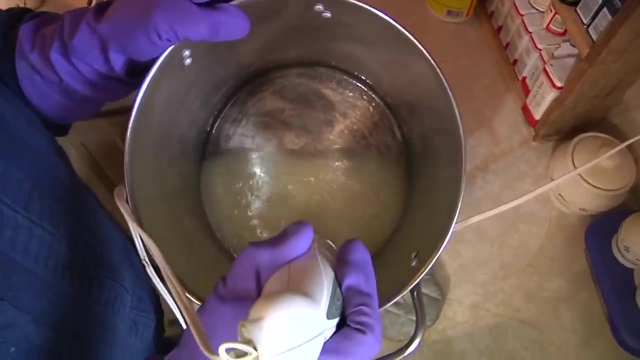 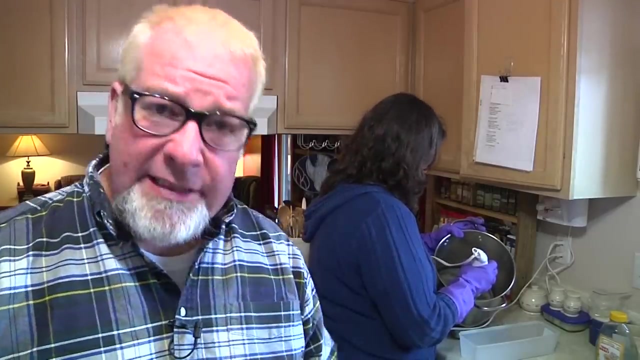 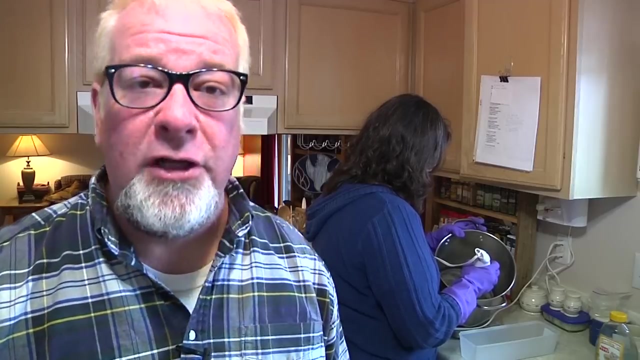 Here we go. Yeah, You see it starting to change there. That is starting to suponify. Okay Now, as my wife is over there blending hard away, right, Basically, I wanted to let you know that if you're doing this with a spoon, if you're just if you don't have a stick blender and you're doing it with a spoon, it does take a little bit of time, about 20 minutes in fact- but the stick blender really cuts that down to about five. 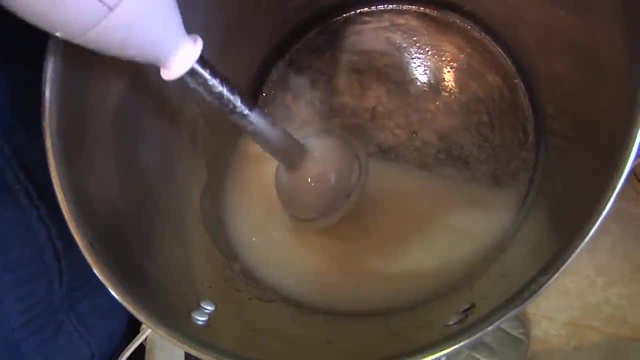 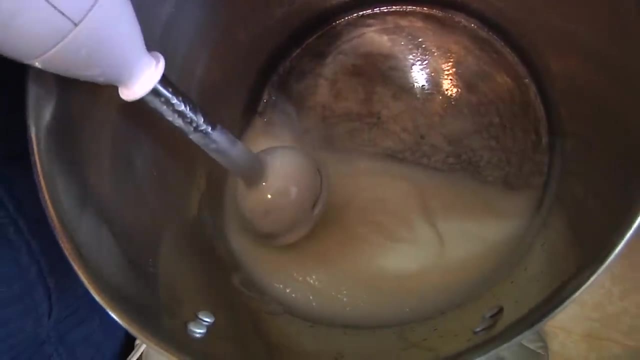 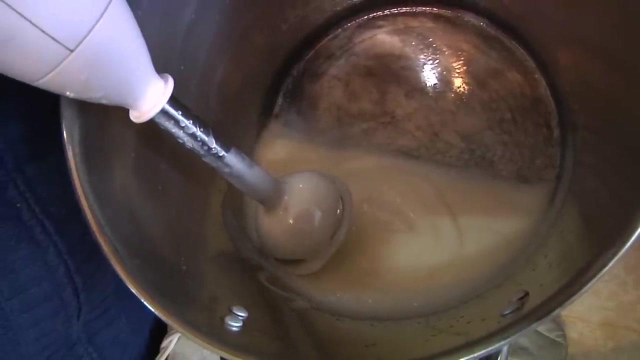 So there's your note, All right. So we've been going about five minutes And I Think you can see trace, you see how it's kind of leaving that mark. the viscosity of this stuff has changed and it's it's like a thin pudding, maybe even- yeah, like a thin pudding rather than a viscous liquid, a very liquidy, watery liquid. 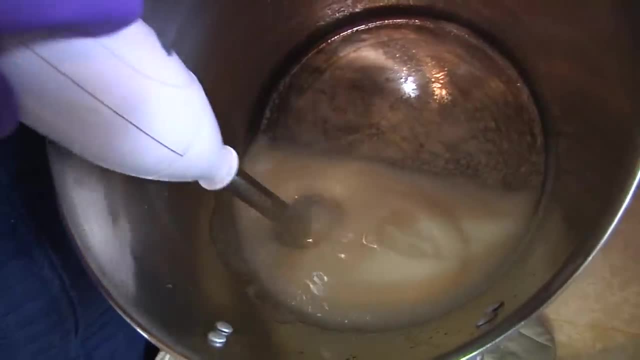 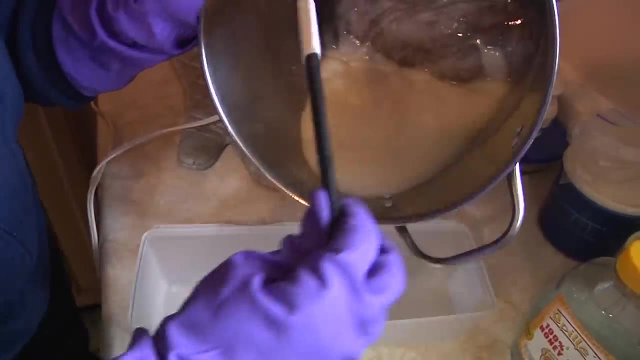 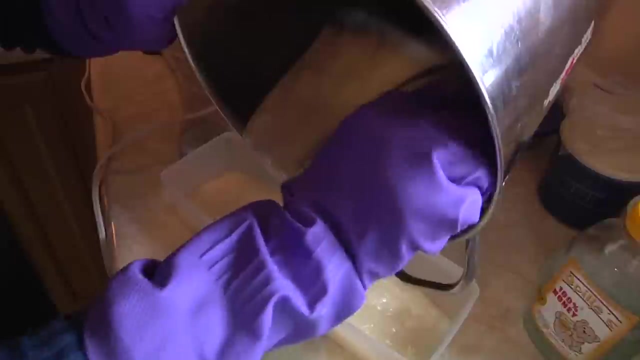 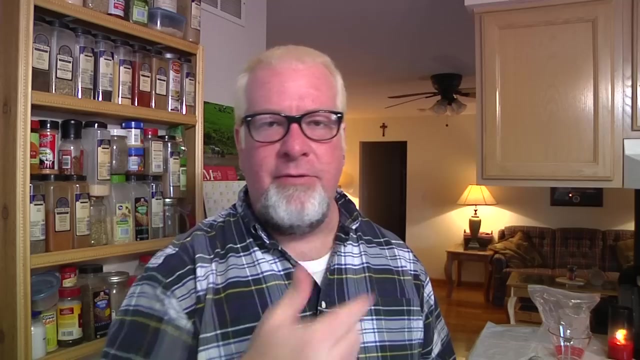 This is now almost soap, And I'll tell you why it's almost soap. right after we pour it into our mold. In you go soap or almost soap, And I'll tell you why in a sec, All right people. So what we have worked and strived and labored, enslaved for whatever- that was five minutes or whatever, uh- is almost soap, almost soap. 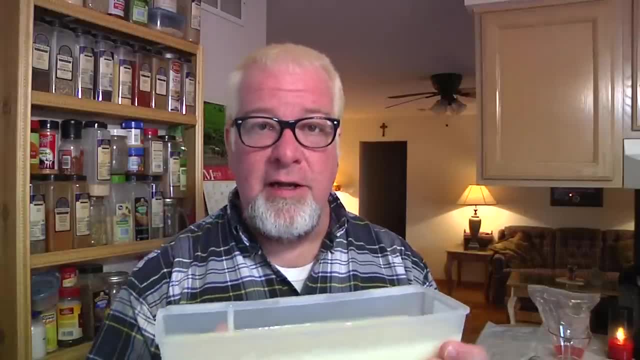 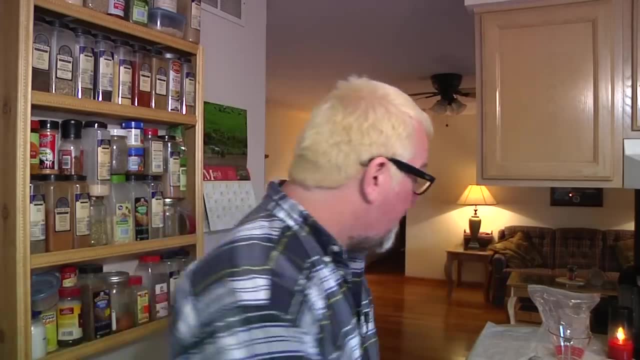 And why is it almost soap? Because it's not soap until the chemical process is complete, And that includes curing. It has to have time to cure. Now, what you're going to do is you're going to take that mold And you're going to set it somewhere for 24 hours. 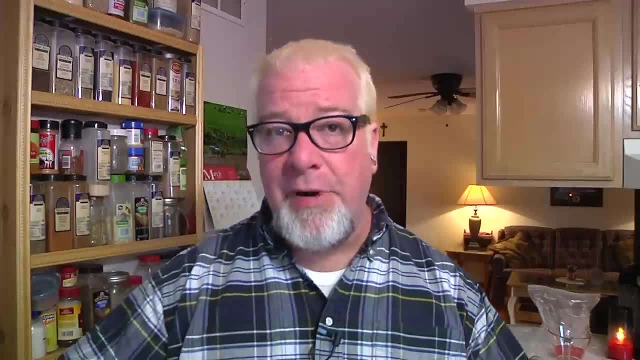 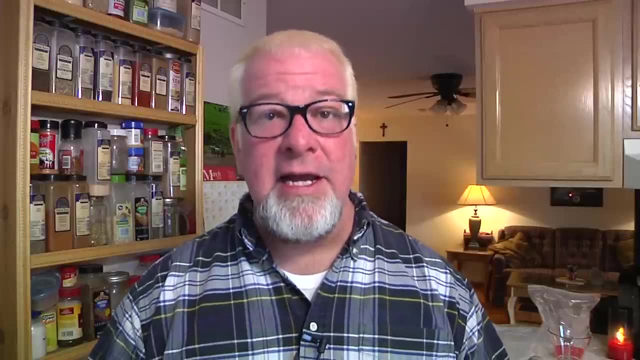 And you're just going to leave it alone, not going to mess with it 24 hours. You're going to pop it out of your mold and you can cut it up at that point if you like, which is really wise, because if you let it cure all the way, it's hard to cut. So you're going to cut it after 24 hours, Then you're going to leave it. It's still not So don't use it. It's still not, So basically going to leave it for about 30 days to completely cure dry, yada yada, yippy skippy.